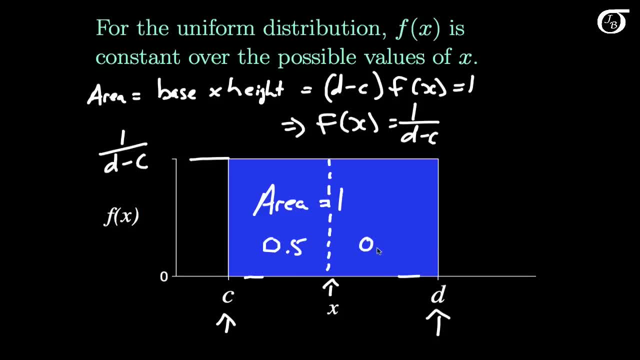 with half the area to the left and half the area to the right. Well, not too hard to see here for the uniform distribution, that that is simply going to be the midpoint between c and d, And since this is a symmetric distribution, the mean and median are equal. 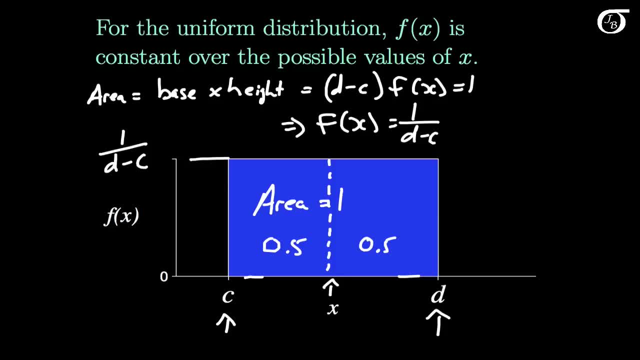 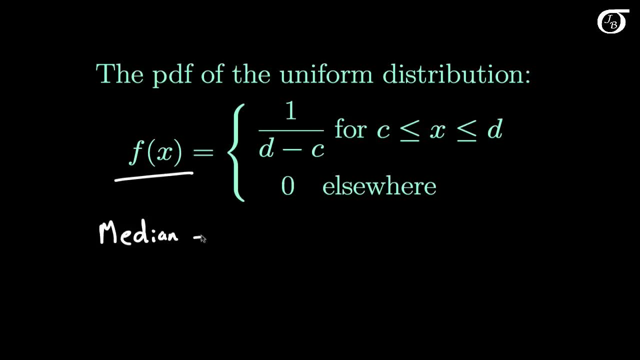 So the mean and median are both equal to the midpoint between c and d. The median is the midpoint between c and d, which simply works out to c plus d over 2.. And the mean, which I'm going to call mu here. 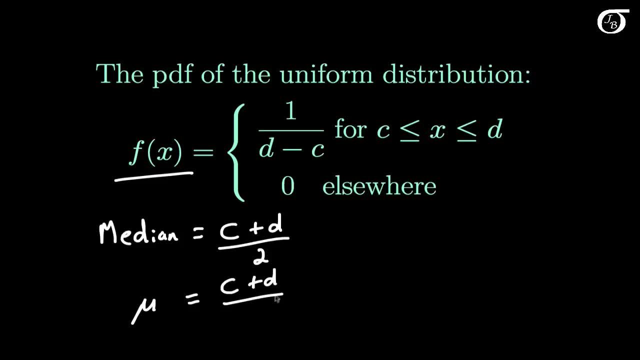 is also equal to that. The midpoint between c and d are just the average of c and d, The variance. we have to use a little calculus to find that, So I can let you verify for yourselves that that is simply equal to 1 over 12 times d minus c squared. 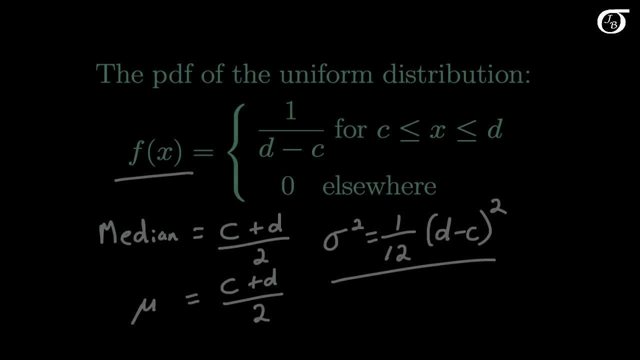 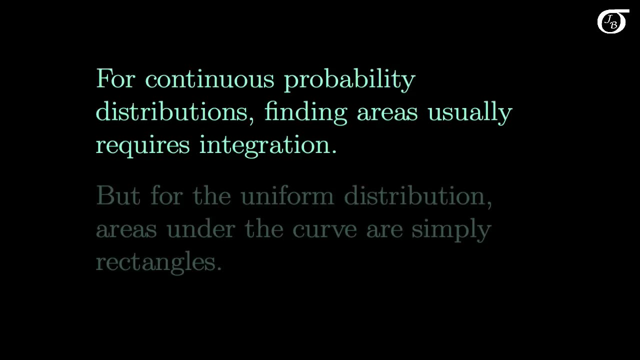 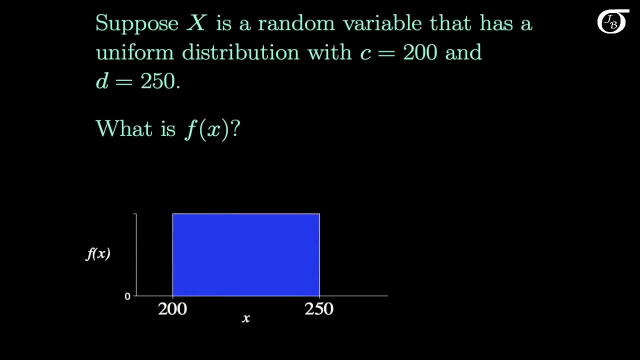 We need to use a little integration to find that For continuous probability distributions, finding areas under the curve usually requires integration, But for the uniform distribution areas under the curve are simply rectangles. So we can find that using simple areas of rectangles. We could use integration if we so desired, but we don't have to. 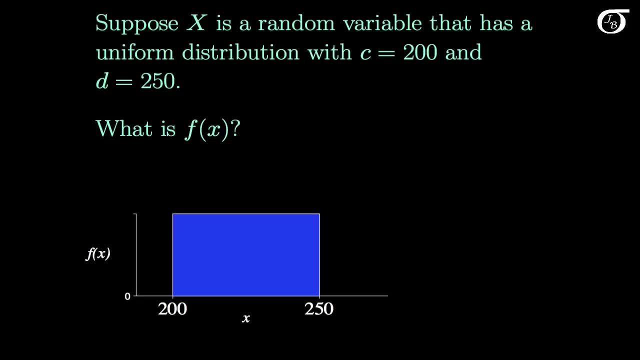 Suppose x is a random variable that has a uniform distribution, with c equal to 200 and d equal to 250.. What is f? f is equal to 1 over d minus c, which is 1 over 250.. 250 minus 200, or 1 over 50.. 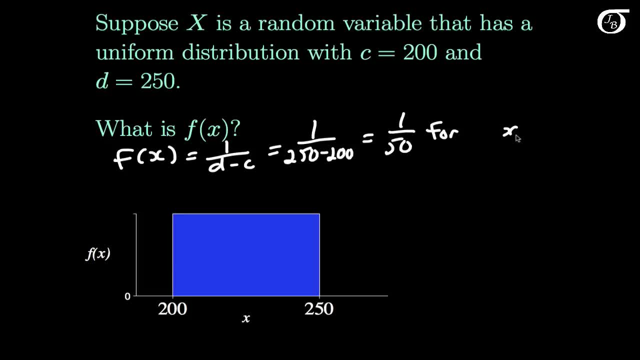 That's not true everywhere, though. that's only true for values of x that lie between 250 and 200. Outside of that interval of values it's equal to 0. So we say f equals 0. otherwise, Visually, what's happening down here is that this height here we just found to be 1 over 50.. 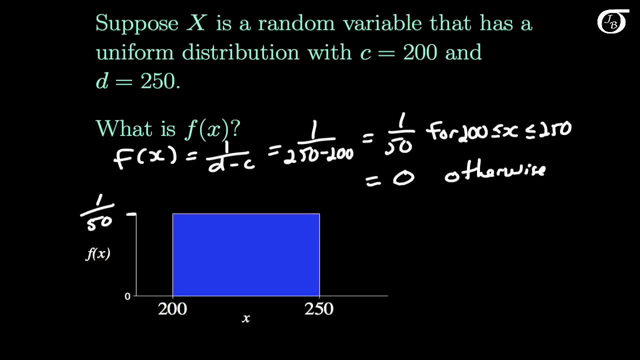 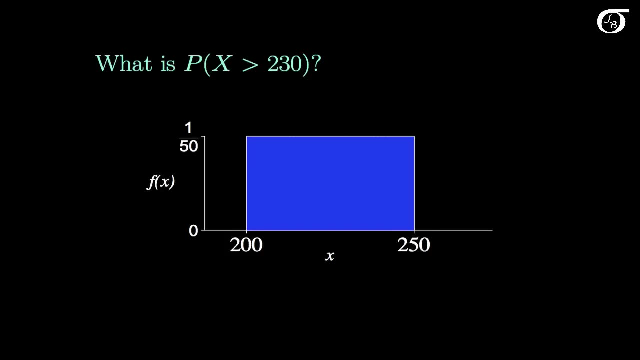 And that makes sure the area under the entire curve is 1.. Outside of 200 to 250, f drops down to 0.. What is the probability the random variable x takes on a value greater than 230?? For continuous random variables, probabilities are areas under the curve.